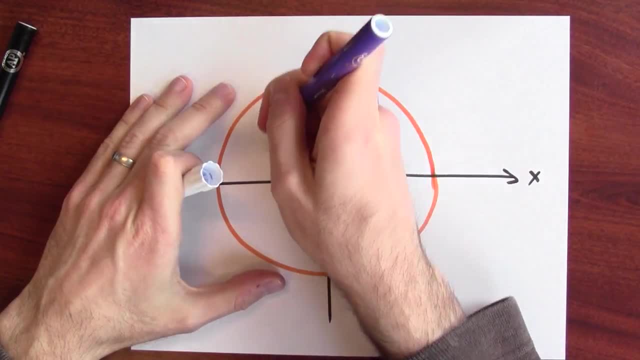 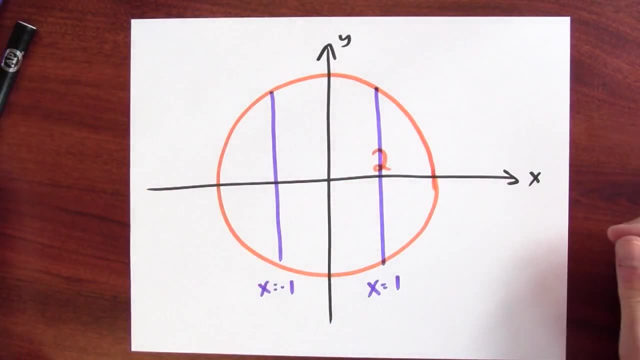 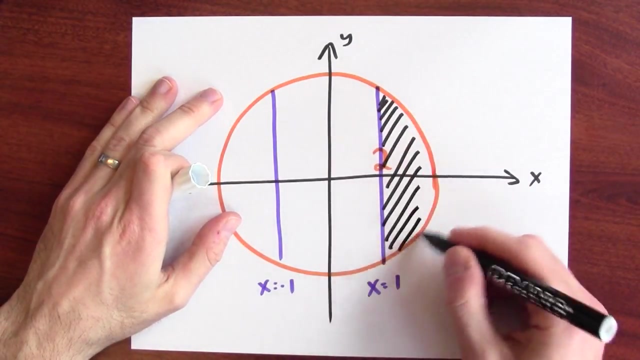 So to do that, let me draw these vertical lines here. This is the line x equals 1,. this is the line x equals minus 1.. Okay now, if I just take the the region in here and rotate it around the y-axis, 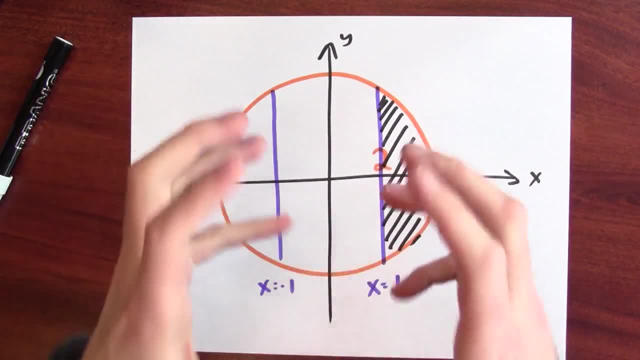 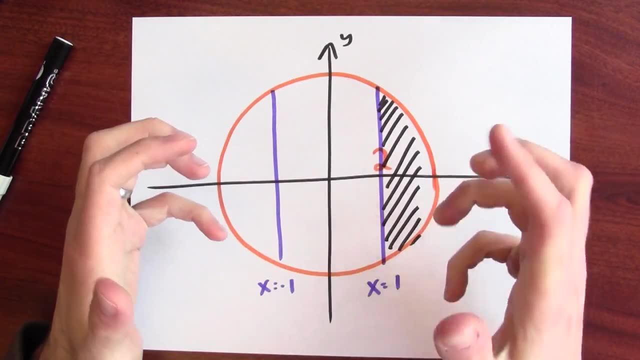 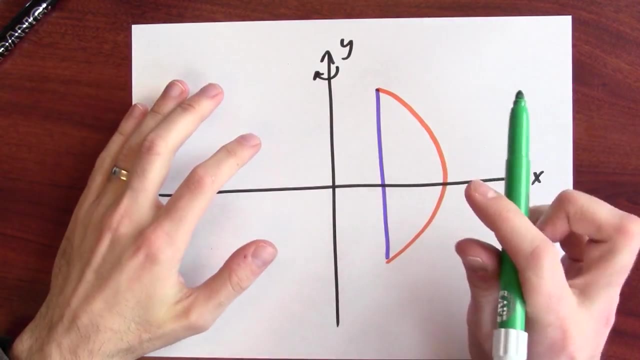 that gives me a bead. It's the same thing as giving me a sphere with a hole drilled out around the y-axis. We've got a choice: We can attack this problem with shells or with washers. Now, if I want to do it with washers, since I'm rotating around the y-axis, I'd 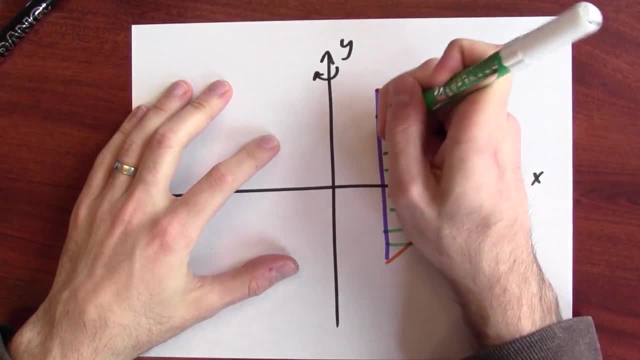 be cutting this into horizontal strips, Because if I take one of these horizontal strips and rotate it around the y-axis, that gives me a washer Okay. so now I've got a bead And I'm going to draw a circle of radius two in the 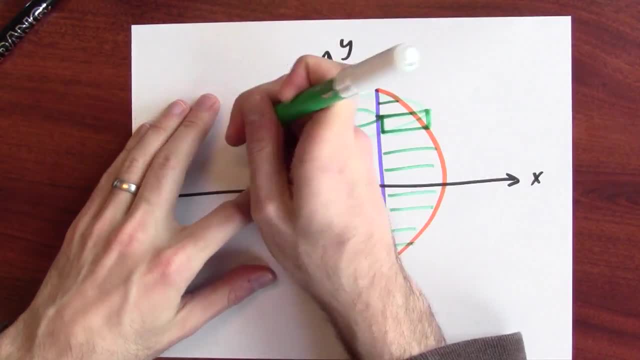 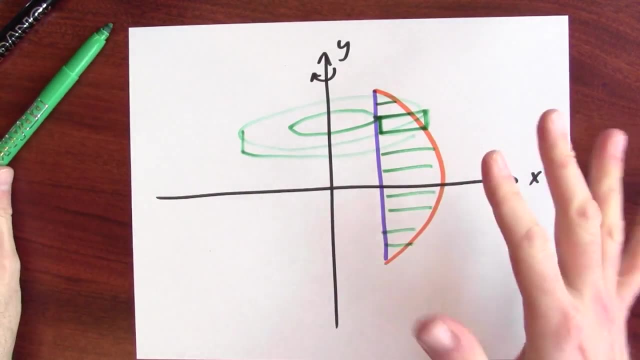 center right. That looks like: here is my here's, here's my big washer, And that's that works, There's. there's nothing wrong with that. But it turns out that if you do it that way, the integral that you get is kind of yucky. 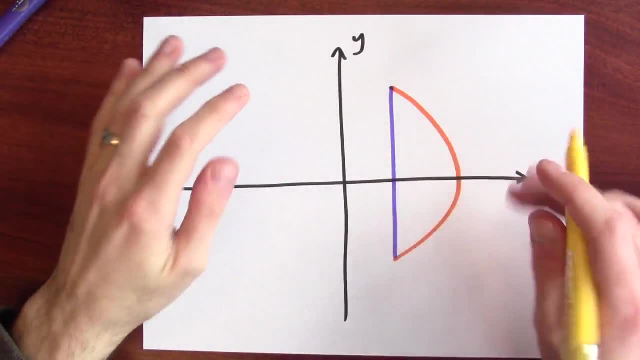 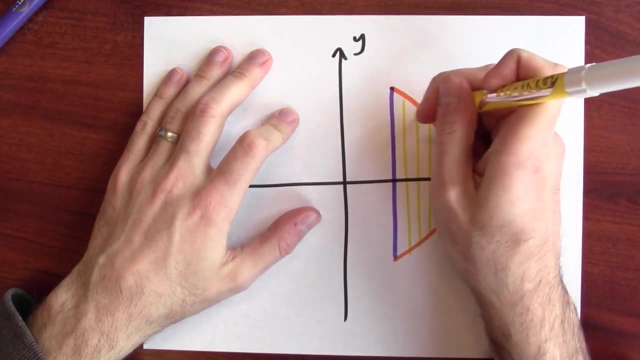 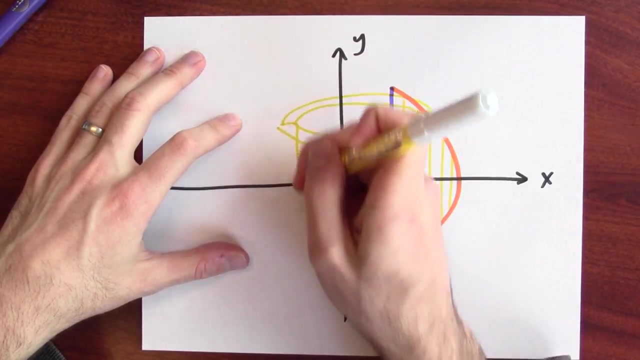 But let's try it instead with shells. If I go with shells, then I'd be cutting this into vertical strips parallel to the axis of rotation, And when I take one of those little vertical strips and rotate it around, well then exactly what I've got right is is one of these shell pieces. 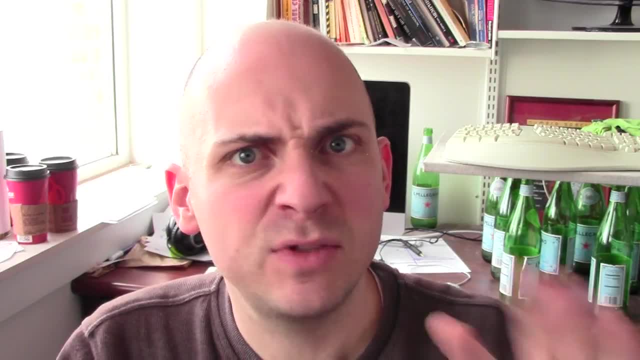 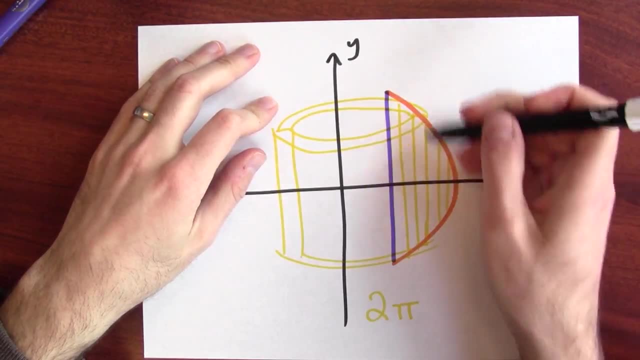 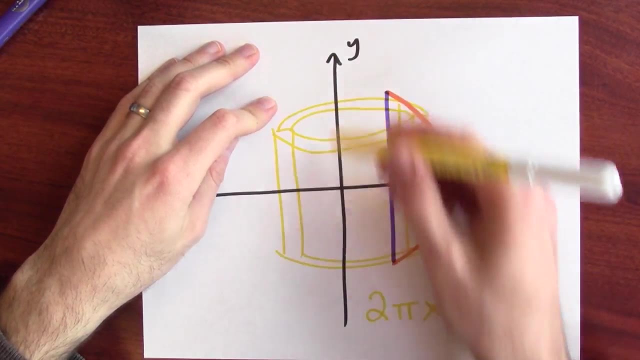 Now we invoke the formula for a volume of a shell in terms of dx. So the formula is 2 pi, the radius of the shell, which, if I think of just one of these pieces, say: at x, the radius is x, since that's how far it is from the axis. 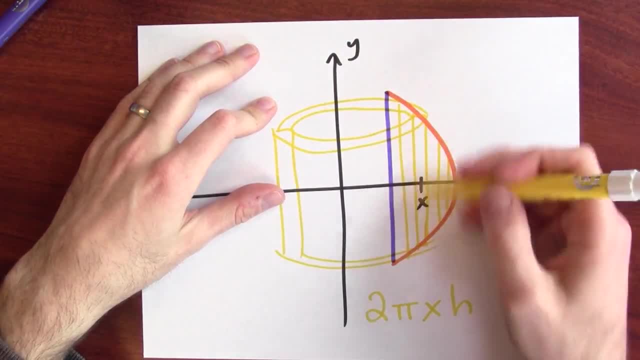 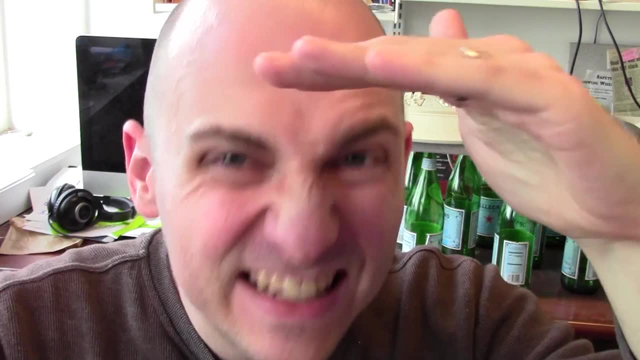 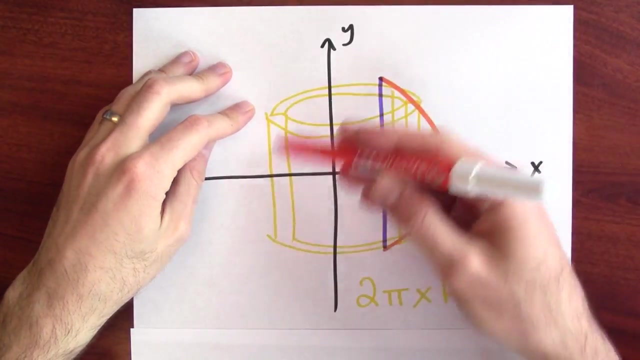 of rotation. The height of the shell, which I haven't figured out yet, Times the thickness of the shell Which is then dx. Now I need to determine the height of the shell So that big sphere has radius 2.. And this orange curve is that circle with radius 2, so I can write down that that. 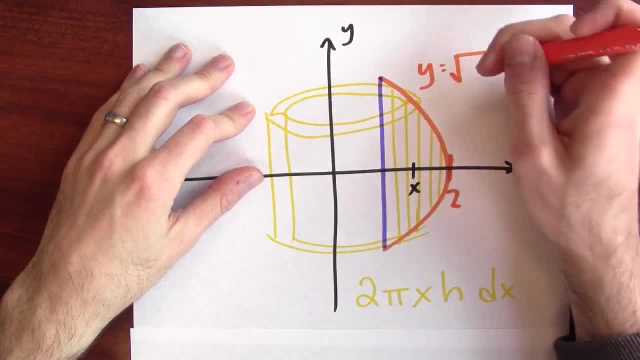 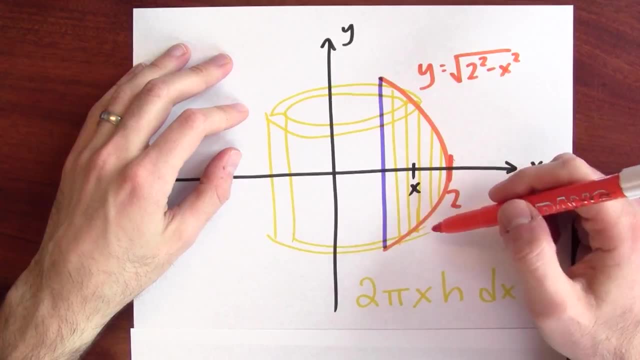 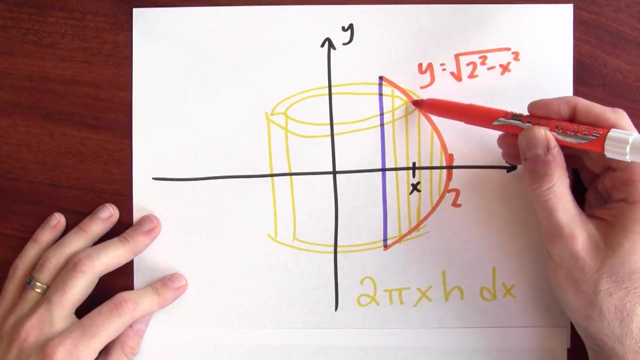 orange curve is: y equals the square root of 2 squared minus x squared, And that's almost enough information to tell me the height of the shell. Let me write down What the height of the shell is then. The height of the shell is well how tall. 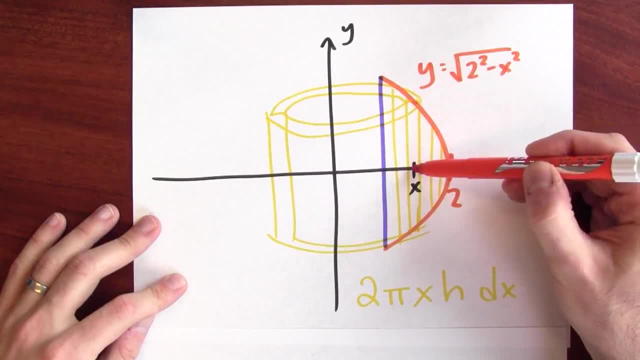 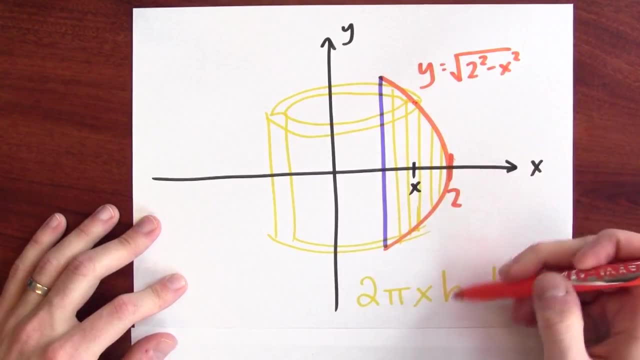 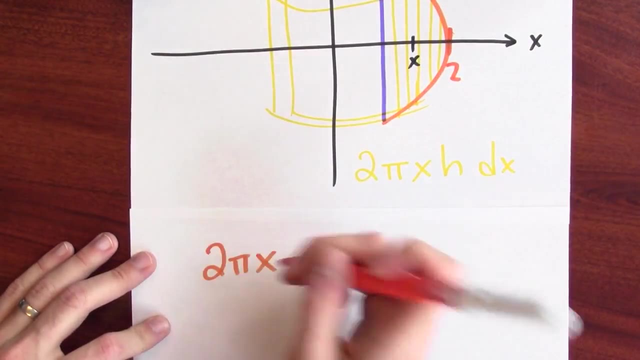 is this thing? Well, here, from here to here, is the square root of 2 squared minus x squared, And then it's the same distance down to the other side here. So the height is twice this quantity. So I can write that down: 2 pi x times the height of the shell. 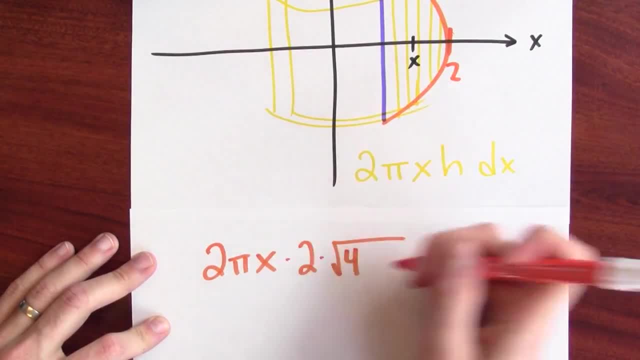 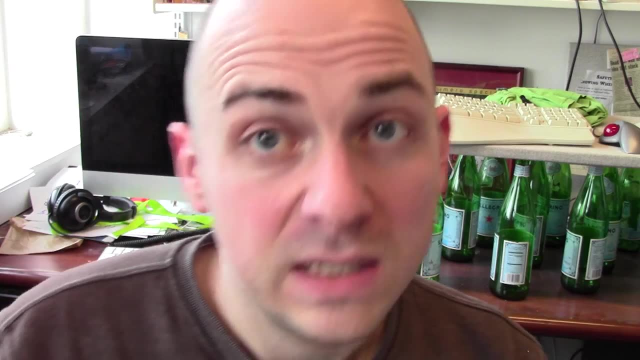 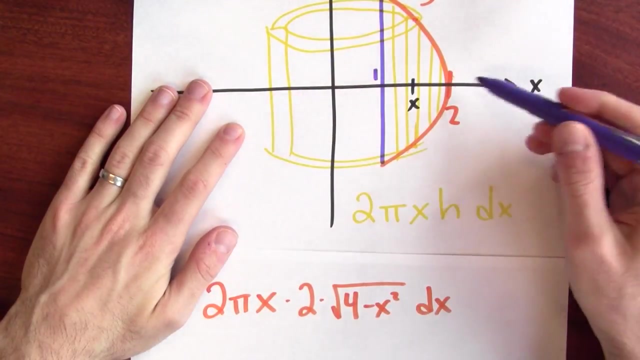 which is 2 times the square root of 2 squared, which is 4, minus x squared. That's the height of the shell And then the thickness of the shell, dx. Let's think about the end points of integration. This purple line right was the line x equals 1.. 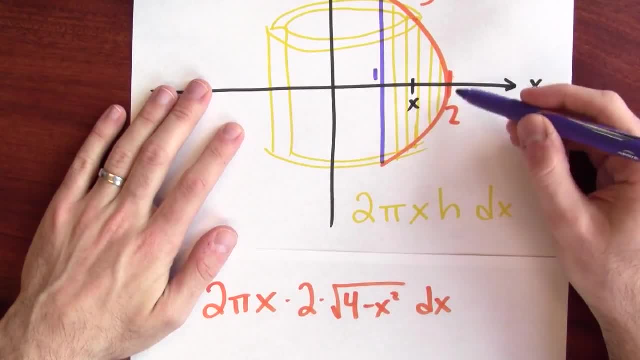 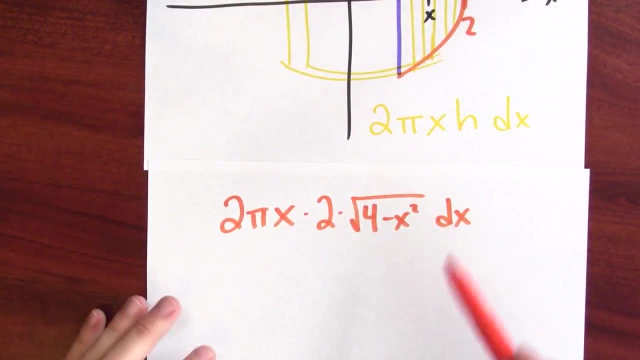 And the orange circle right has radius 2.. So x can take values between 1 and 2.. And that tells me what my end points of integration should be. So this is the volume of just one of those shells And I'm going to integrate that. 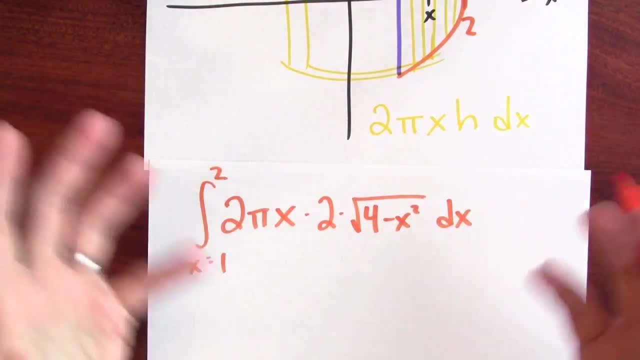 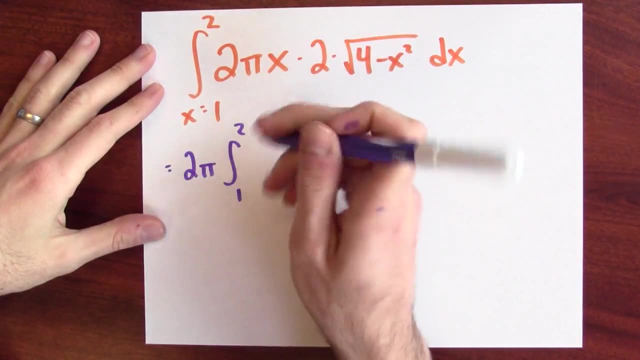 X goes from 1 to 2 to get all of the shells and add them all together. Finally we integrate. This is 2 pi times the integral from 1 to 2.. And I'll write 2x, the square root of 4. 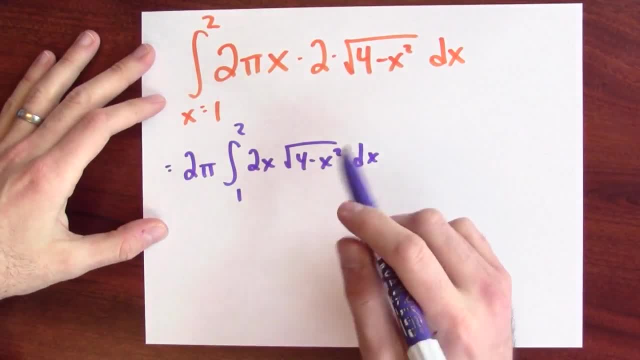 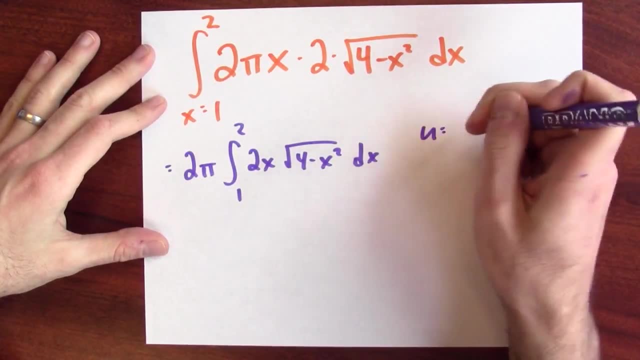 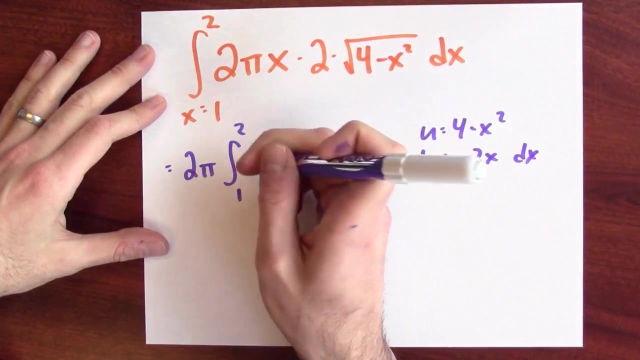 minus x squared dx, And this is really where shells shine. I set this up now and you can see I can make a? u substitution here, So I'll set u equal 4 minus x squared. du in that case is minus 2x dx. 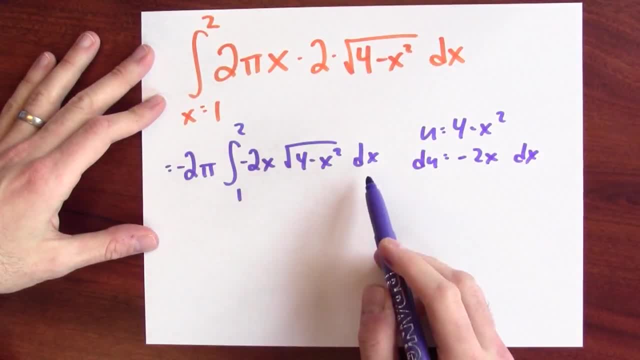 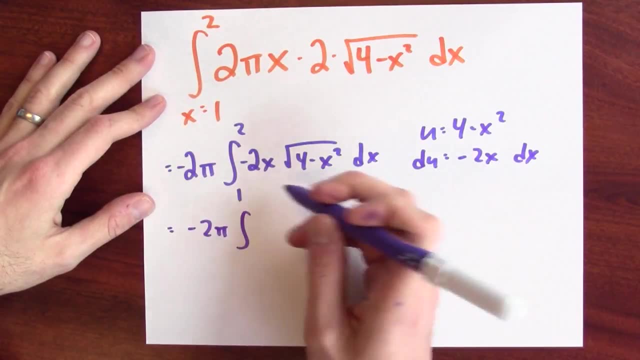 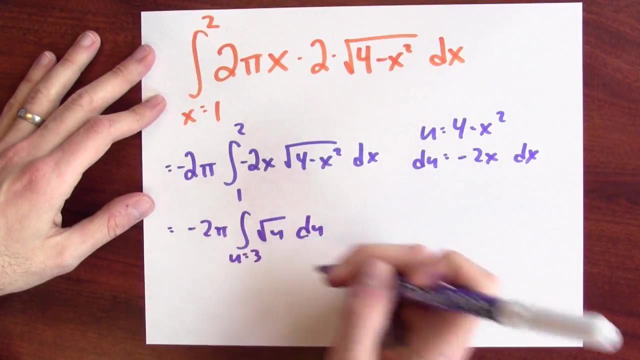 Put a minus sign there and a minus sign there. Now I've got du square root of u, So this integral becomes minus 2 pi square root of u, du, And I can change the end points. u goes from: when x is 1, u is 3.. When x is 2, u is 0.. 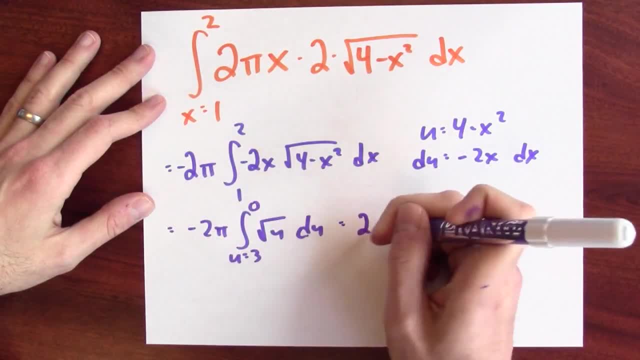 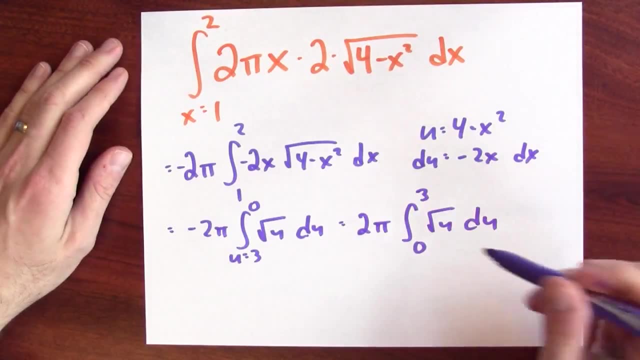 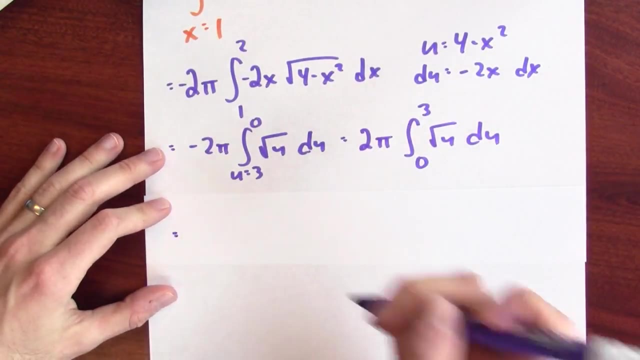 And this is negative- from 3 to 0. So I can rewrite this as 2 pi, the integral from 0 to 3 of the square root of u du. Now, that's not hard to do, right? I can rewrite that, that integrand, as 2 pi. 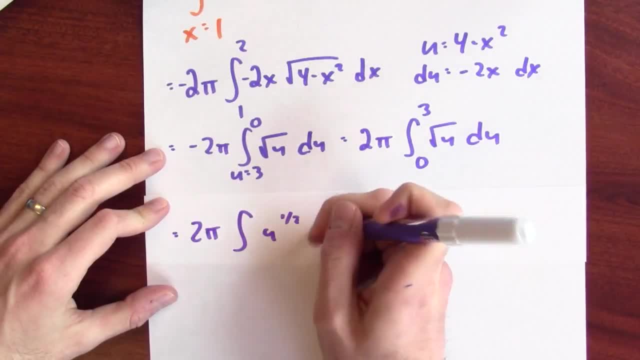 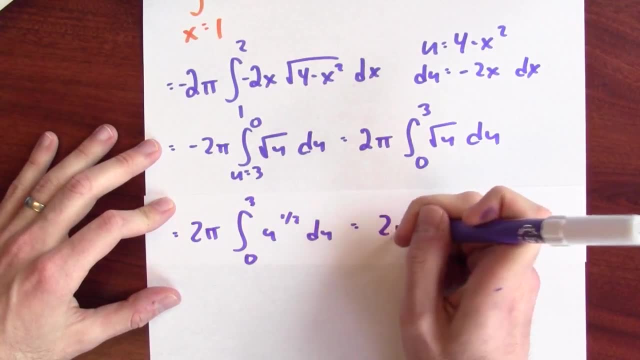 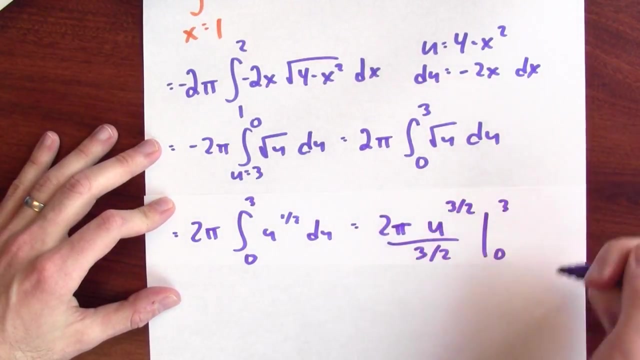 the integral of u to the 1 half du from 0 to 3.. And now I can easily anti-differentiate that using the power rule. So this is 2 pi u to the 3 halves over 3 halves, evaluated at 0 and 3.. 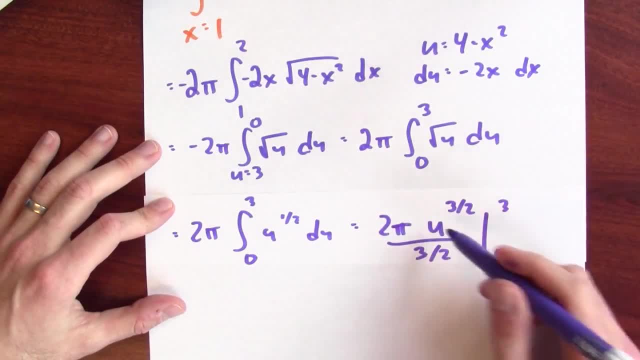 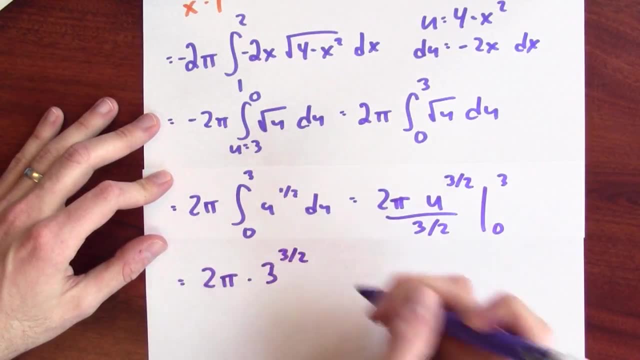 Now when I plug in 0, I just get 0. So my answer is: whatever I get when I plug in 3.. So the volume is 2 pi times 3 to the 3 halves power over 3 halves. Now, instead of writing 3 to the 3 halves power, I could write this as 2 pi over 3. 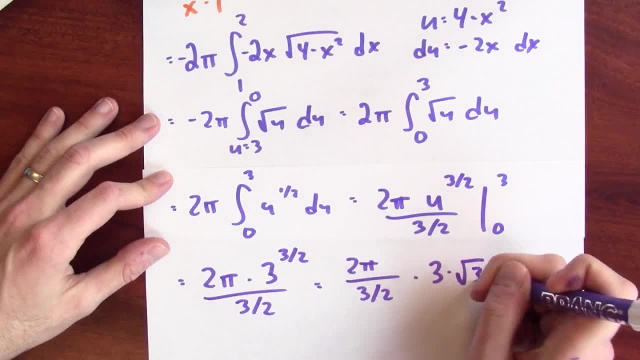 halves times 3 times the square root of 3, right, That's the same as 3 to the 3 halves power. But look, this 3 and this 3 cancel, and I'm dividing by a half here. So this ends up being: 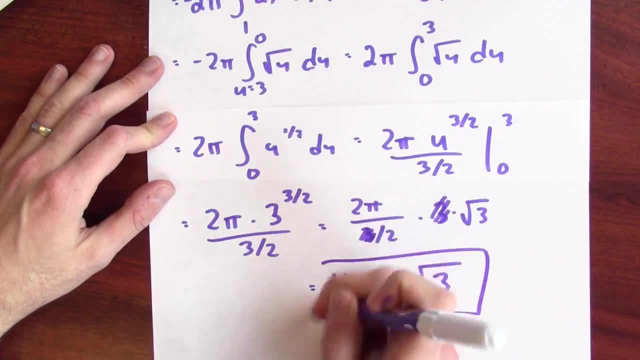 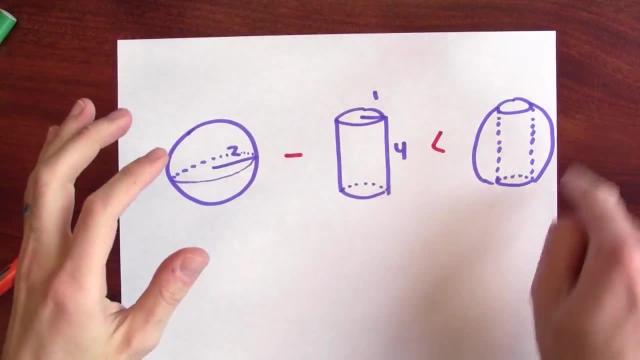 4 pi times the square root of 3.. This is the volume of our bead. We did it, But is the answer reasonable? Well, to think about how reasonable our calculation for the volume of the bead was, we could think about how we built the bead right. 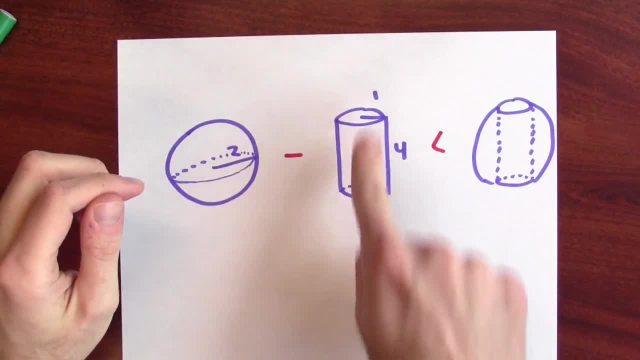 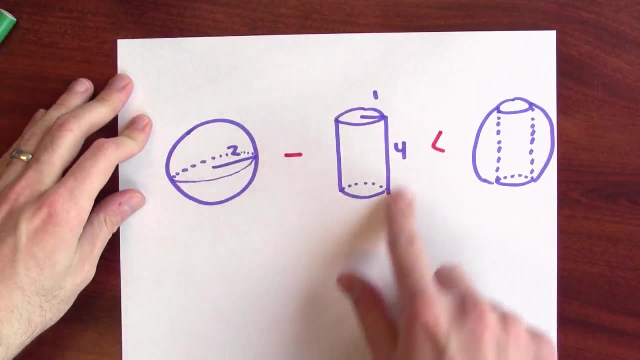 We built this thing by starting with a sphere of radius 2 and then drilling out a tube of radius 1.. So if I start with a sphere of radius 2 and I subtract even more volume right, This cylinder of height 4 extends above. 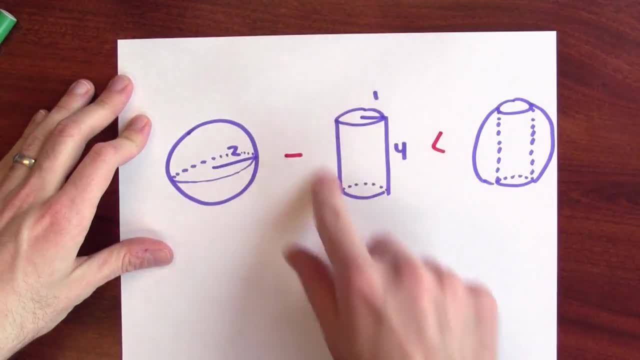 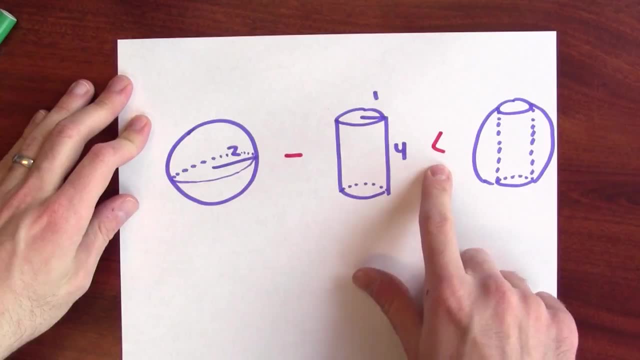 the top of the sphere and below the bottom of the sphere. So this is even more material than I removed to get the bead. Well, that means that the volume of the sphere minus the volume of the cylinder has got to be even a little bit less than the volume of the bead right. 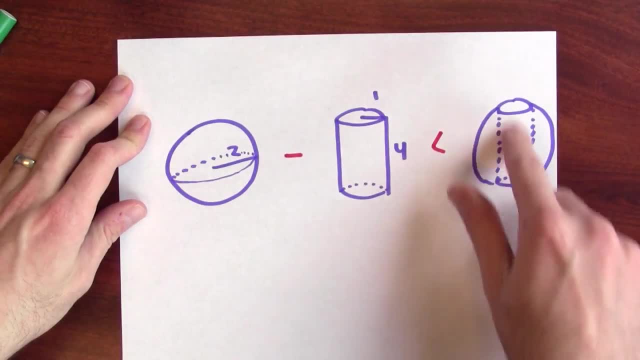 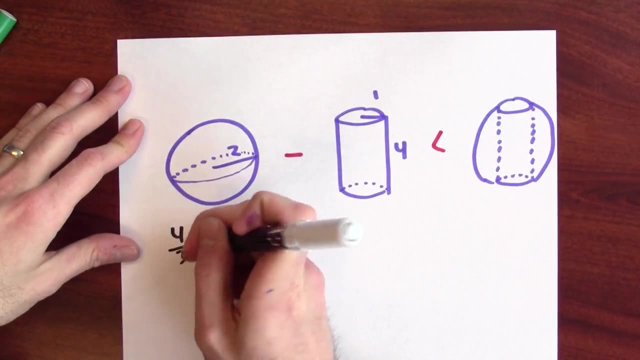 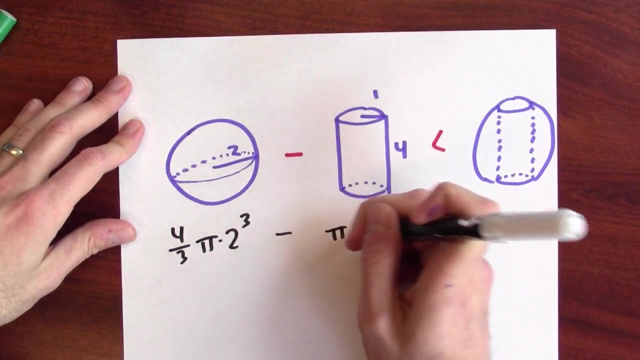 Because this is a little bit more material than the material that we removed to get the bead. Well, how big are these three things? This thing here is 4 thirds pi radius cubed. that's the volume of a sphere. And this, this thing here is pi r squared times height, is the volume of the. 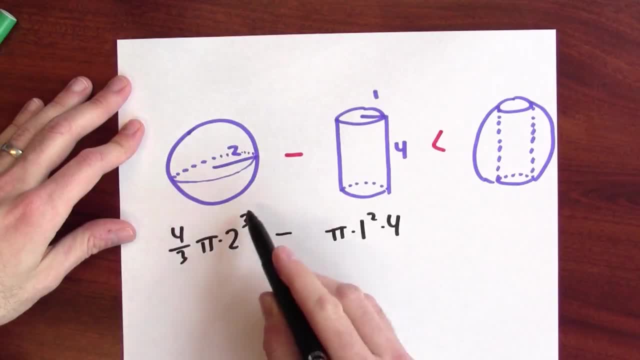 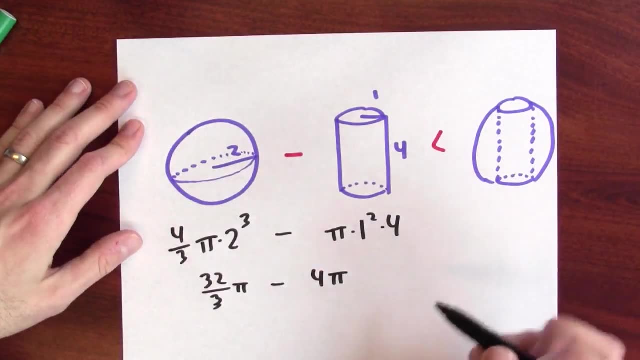 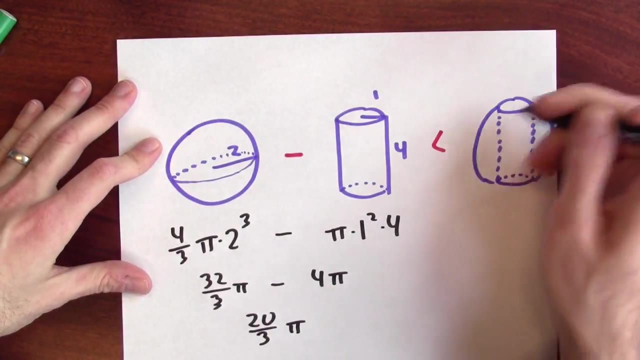 cylinder. I could simplify this a bit. This is 4 times 8, so that's 32 thirds pi minus 4 pi. And I could simplify that a little bit further. even That's 20 thirds pi. And where do we get to the volume of the?